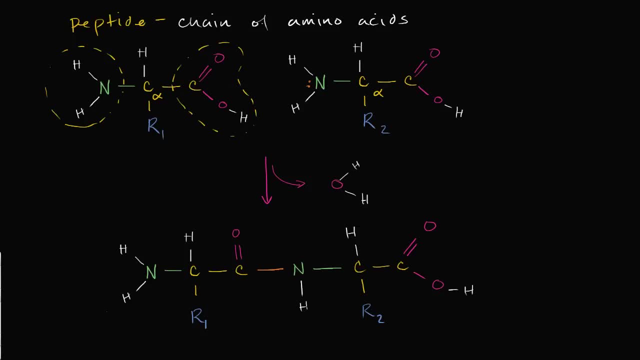 to form a bond with this carbonyl carbon right over here. So this lone pair goes to this carbonyl carbon, forms a bond, and then this hydrogen. this hydrogen, this oxygen, could be used net-net to form a water molecule. 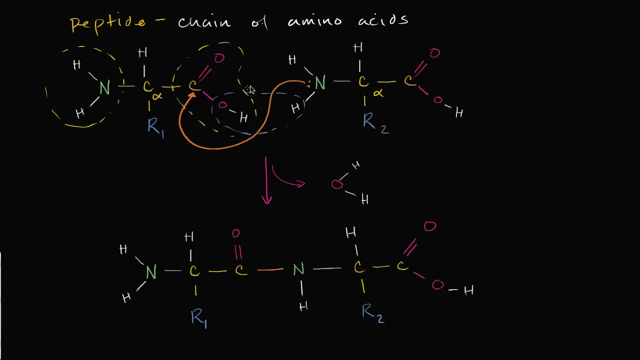 to form a water molecule that's let go from both of these amino acids. So this reaction: you end up with the nitrogen being attached to this carbon and a release of a water molecule. And because you have the release of this water molecule, this type of reaction- we've seen it many other times. 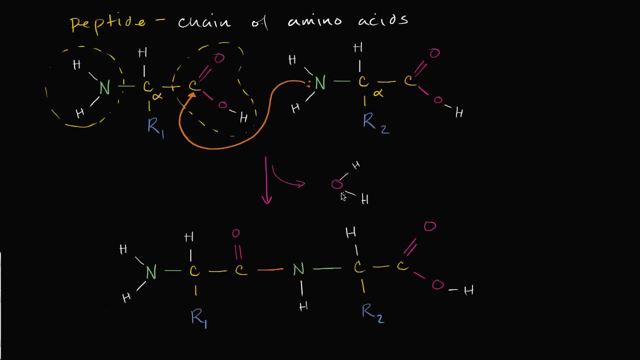 in other types of, with other types of molecules. we call this a condensation reaction or dehydration synthesis. So con condensation, condensation reaction, Or or dehydration synthesis- Dehydration: we saw this type of reaction where we're putting glucoses together. 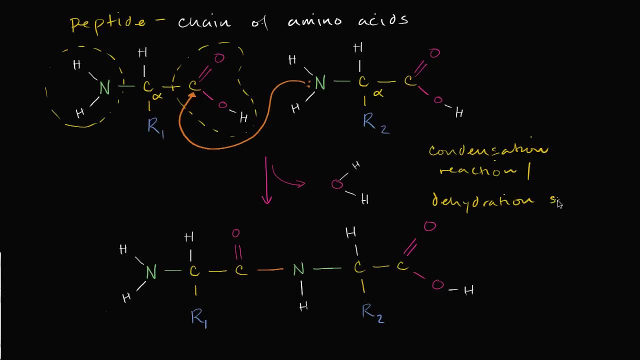 when we were forming, when we were forming carbohydrates, Dehydration, dehydration, synthesis. But whenever I see a reaction like this, it's somewhat satisfying to just be able to do the counting and say, all right, this is gonna bond with that. 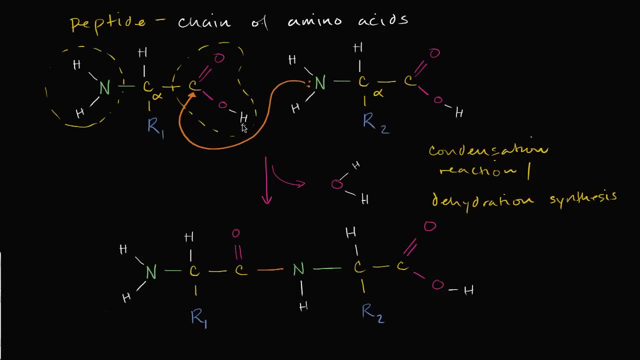 this is gonna bond right over there. I have and I'm gonna let go of an oxygen and two hydrogens, which net-net equals H2O, equals a water molecule. But how could we actually imagine this happening? Can we push the electrons around? 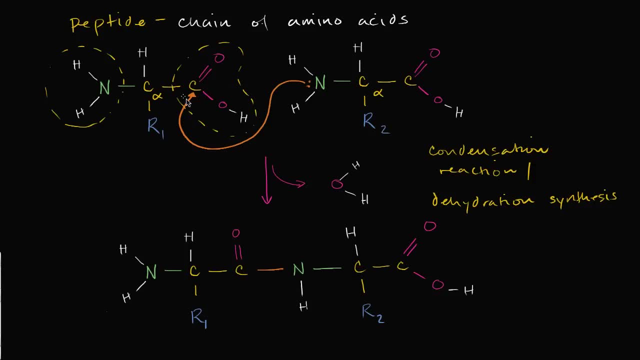 Can we do a little bit of high-level organic chemistry to think about how this happens? And that's what I wanna do here. I'm not gonna do a kind of a formal reaction mechanism, but really get a sense of what's going on. 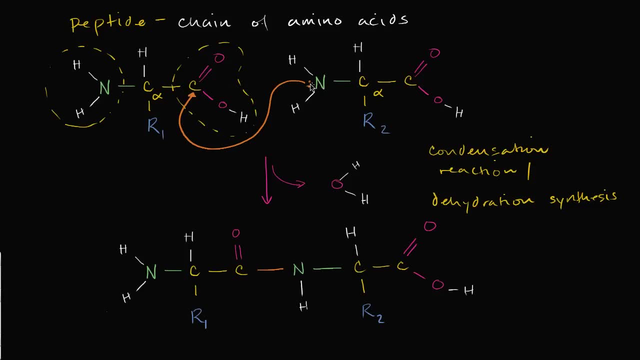 Well, nitrogen, as we said, has got this lone pair. It's electronegative And it and this carbon right over here. it's attached to two oxygens. Oxygens are more electronegative. The oxygens might hog those electrons. 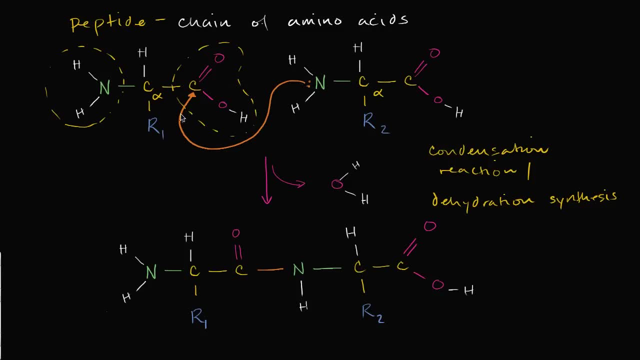 And so this nitrogen might wanna do what we call in organic chemistry a nucleophilic attack on this carbon right over here. And when it does that, if we were doing a more formal reaction mechanism we could say, hey, well, maybe these. 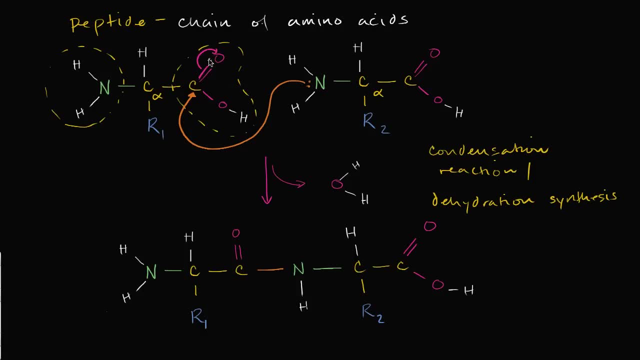 one of the double bonds goes back, the electrons in it go back to this oxygen and then that would have a negative and then that oxygen would have a negative charge. But then that lone pair from that double bond could then reform. it could reform. 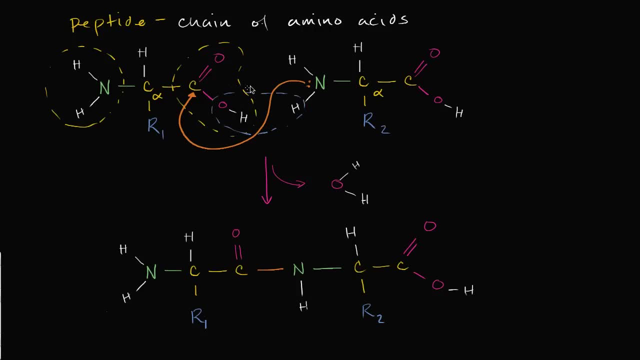 to form a water molecule. that's let go from both of these, from both of these amino acids. So this reaction: you end up with the nitrogen being attached to this carbon and a release, a release of a water molecule. And because you have the release of this water molecule, 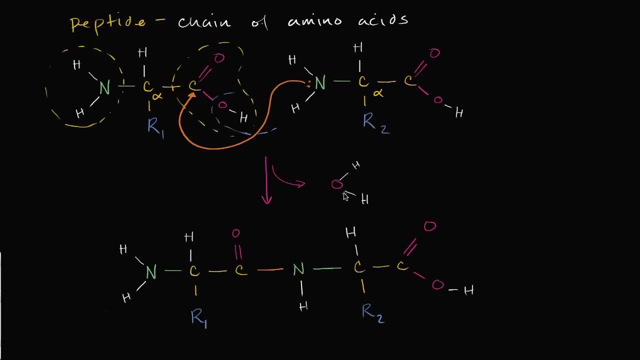 this type of reaction. we've seen it many other times in other types of, with other types of molecules. we call this a condensation reaction or dehydration synthesis. So con condensation, condensation reaction, Or or dehydration synthesis. 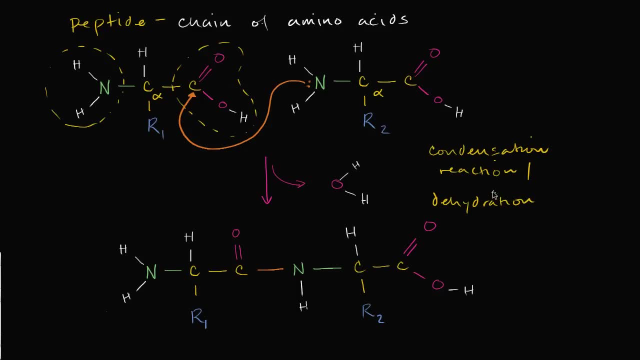 Dehydration. we saw this type of reaction where we're putting glucoses together when we were forming, when we were forming carbohydrates, Dehydration, dehydration synthesis. But whenever I see a reaction like this, it's somewhat satisfying to just be able to do the counting. 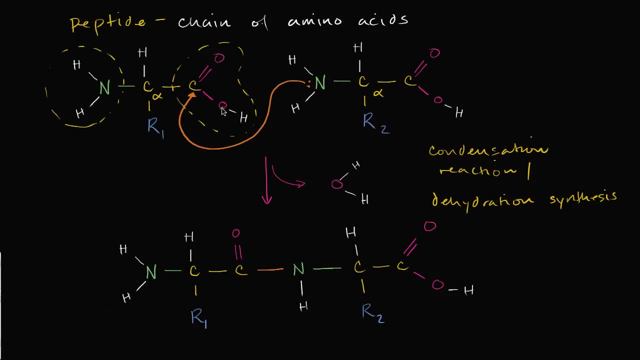 and say: all right, this is gonna bond with that. it's gonna bond. right over there I have and I'm gonna let go of an oxygen and two hydrogens which net net equals H2O, equals a water molecule. 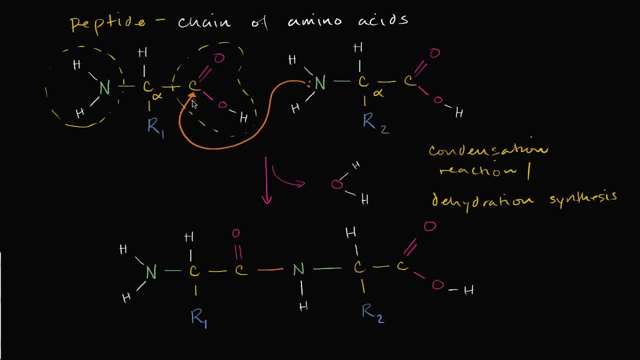 But how could we actually imagine this happening? Can we push the electrons around? Can we do a little bit of high-level organic chemistry to think about how this happens? And that's what I wanna do here. I'm not gonna do a kind of a formal reaction mechanism. 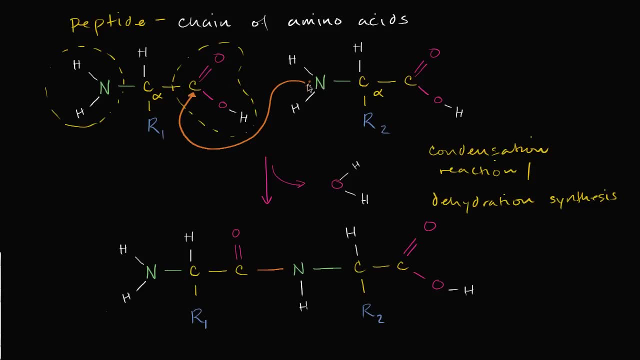 but really get a sense of what's going on. Well, nitrogen, as we said, it's got this lone pair, it's electronegative and it and this carbon right over here. it's attached to two oxygens. 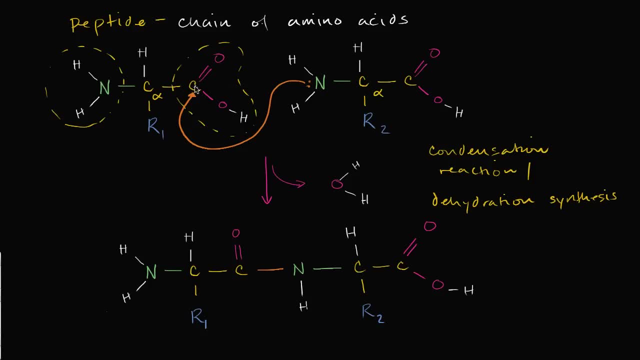 The oxygens are more electronegative. The oxygens might hog those electrons, And so this nitrogen might wanna do what we call in organic chemistry a nucleophilic attack on this carbon right over here And when. it does that if we were doing a more formal reaction mechanism. 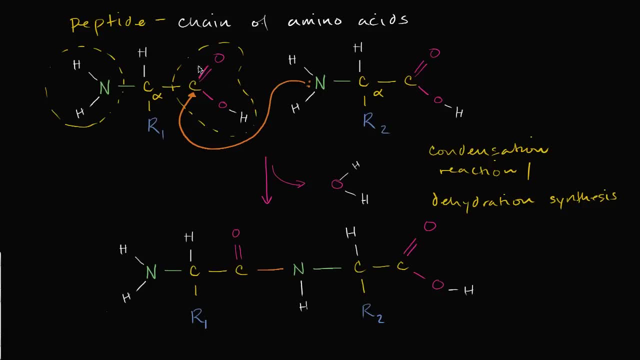 we could say, hey, well, maybe these one of the double bonds goes back, the electrons in it go back to this oxygen, and then that would have a negative and then that oxygen would have a negative charge. But then that lone pair from that double bond. 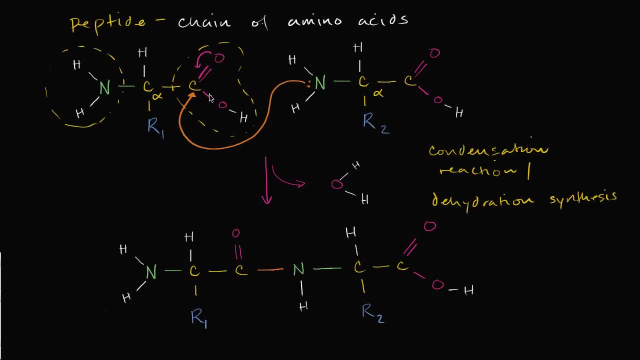 could then reform. It could reform and, as that happens, as that happens, this, this oxygen that's in the hydroxyl group will take back both of these electrons, would take back, would take back both of those electrons. and now it's going to have an extra lone pair. 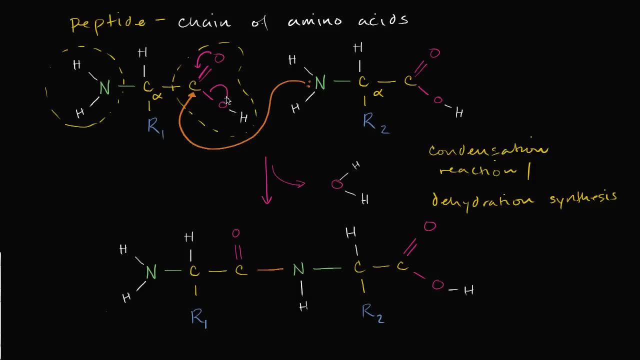 and then, as that happens, as that happens, this oxygen that's in the hydroxyl group will take back both of these electrons, Would take back, would take back both of those electrons And now it's going to have an extra lone pair. 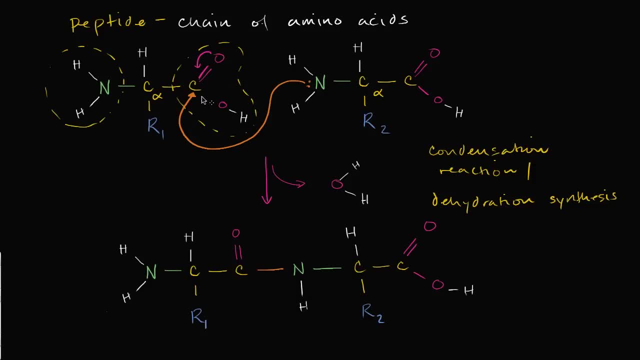 Now it's going to have an extra lone pair, And let me do that by erasing this bond and then giving it, giving it an extra lone pair. It already had two lone pairs. It already had two lone pairs And then, when it took that bond, 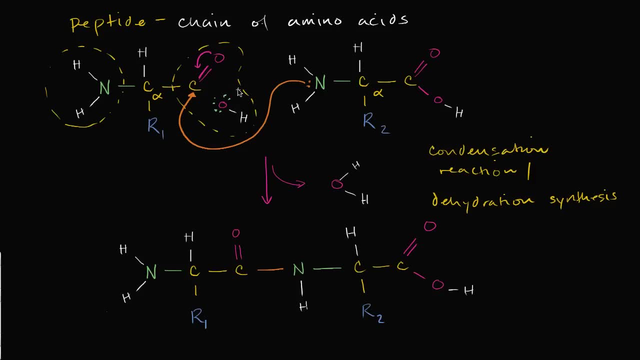 it's gonna have a third lone pair And it's going to have- it's going to have- a negative charge And now you could imagine it's going to grab a hydrogen proton someplace. Now it could just grab any hydrogen proton, but probably the most convenient one would be this one. 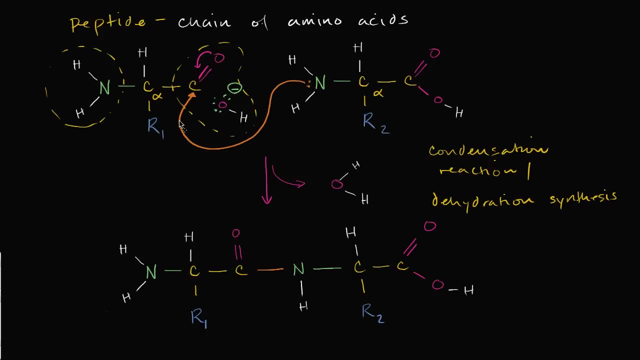 Because if this nitrogen is giving is going to use this lone pair to form a bond with carbon, it's going to have a positive charge and it might want to take these electrons back. So you could imagine where this one of these lone pairs is used to grab. 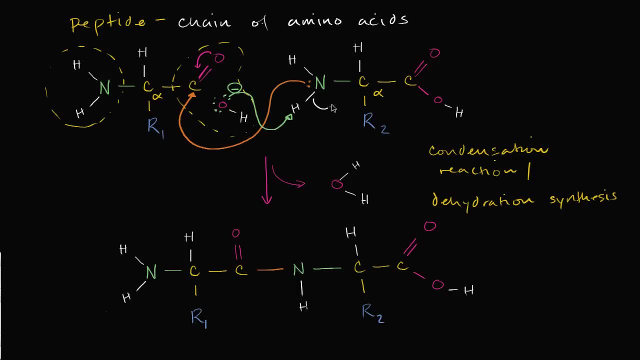 this hydrogen proton and then the nitrogen can take these electrons, can take these electrons back. So hopefully you didn't find this too convoluted, but I always like to think, well, what could actually happen here. And so you see this lone pair of electrons. 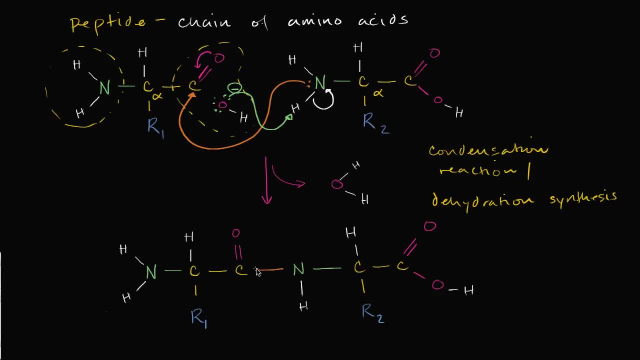 from the nitrogen forms this orange bond. with the carbon. It forms this orange, this- let me do that in an orange color, if I'm gonna call it an orange bond. It forms this orange bond. This is what we call this orange bond. 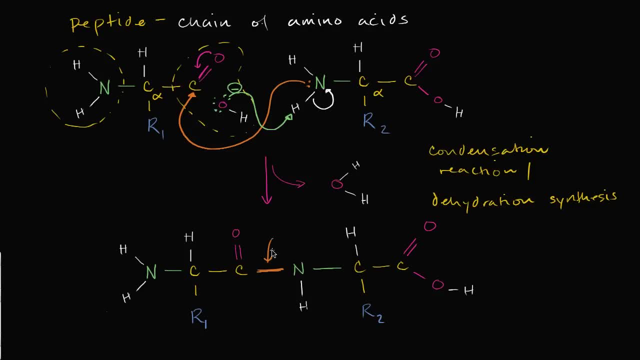 We could call this a peptide bond, So that, or a peptide linkage, Peptide Peptide bond, sometimes called a peptide linkage, And we have, and then we have the release of a water molecule. So you have this oxygen, is this oxygen? 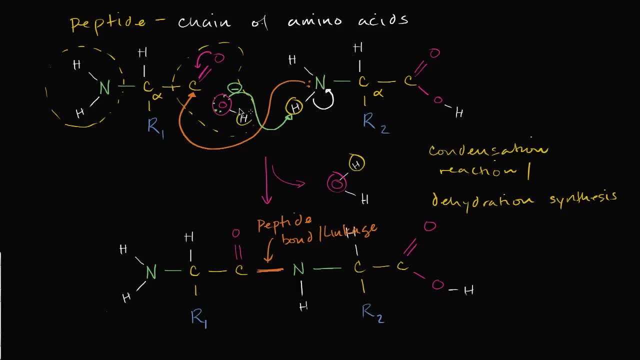 and you could imagine, this hydrogen is this hydrogen and this hydrogen is this hydrogen right over here. And so now that it all works out, Now, when I first saw this reaction I was like, okay, that kind of makes sense, except for the fact that in 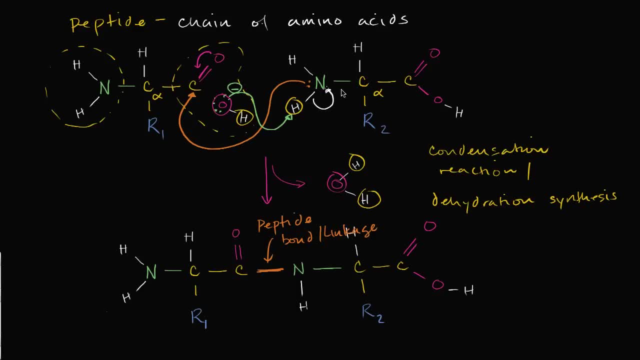 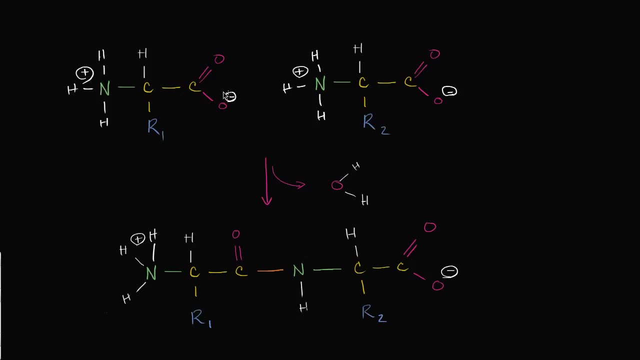 at physiological pHs. amino acids don't tend to be in this form. In physiological pHs, you're more likely- you're more likely to find this form of the amino acids. Define them as zwitterions or zwitterions. 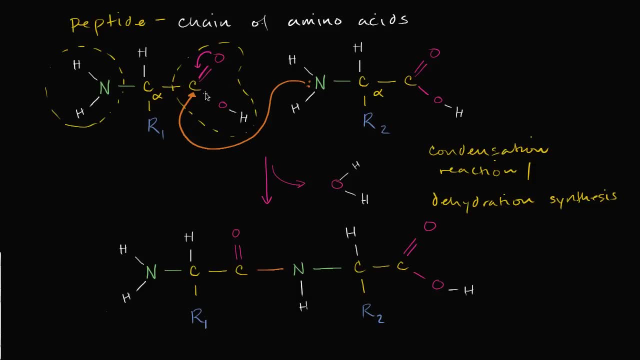 Now it's going to have an extra lone pair, and let me do that by erasing this bond and then giving it, giving it an extra lone pair. It already had two lone pairs. It already had two lone pairs and then, when it took that bond, 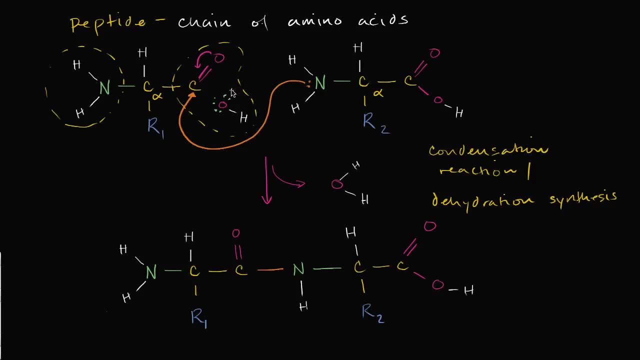 it's going to have a third lone pair and then it's going to have- it's going to have- a negative charge and now you could imagine it's going to grab a hydrogen proton someplace. Now it could just grab any hydrogen proton. 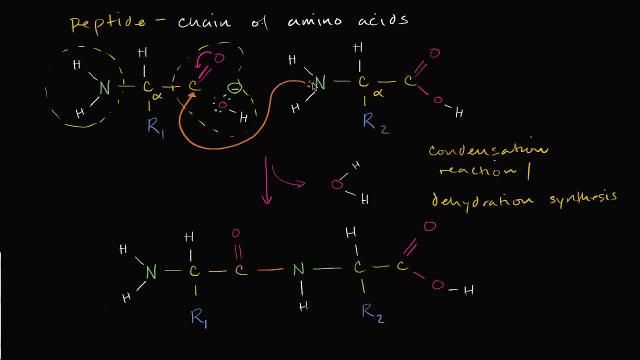 but probably the most convenient one would be this one, because if this nitrogen is giving is going to use this lone pair to form a bond with carbon, it's going to have a positive charge and it might want to take these electrons back. 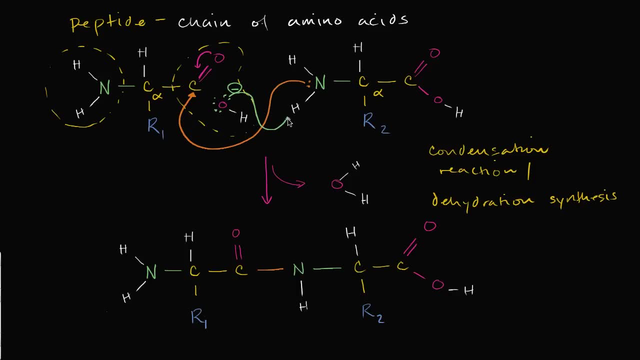 So you could imagine where this one of these lone pairs is used to grab this hydrogen proton and then the nitrogen, and then the hydrogen can take these electrons, can take these electrons back. So hopefully you didn't find this too convoluted. 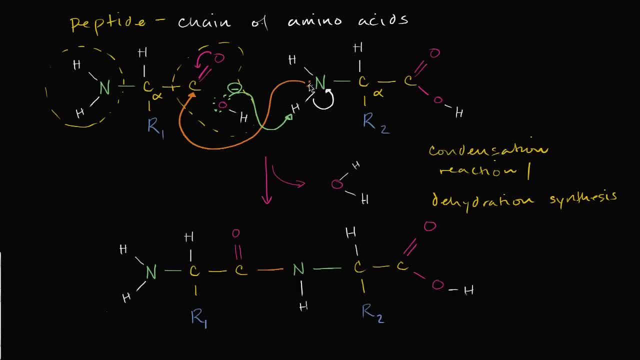 but I always like to think, well, what could actually happen here. And so you see, this lone pair of electrons from the nitrogen forms this orange bond with the carbon. It forms this orange, this. let me do that in orange color. 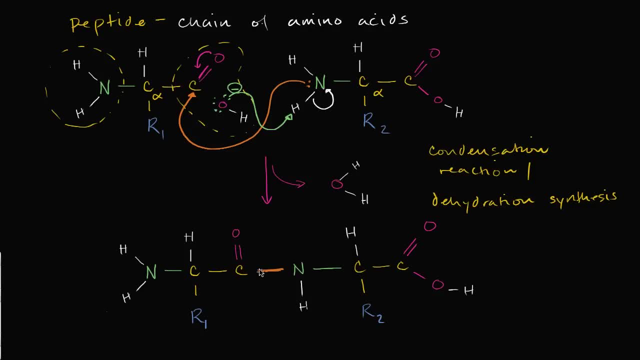 if I'm going to call it an orange bond, It forms this orange bond. This is what we call this orange bond. We could call this a peptide bond, so that, or a peptide linkage, Peptide, Peptide bond, sometimes called a peptide. 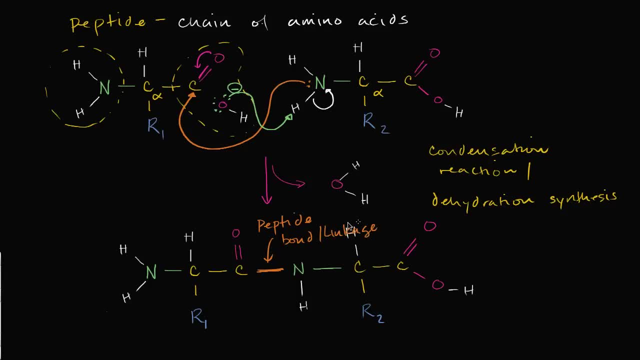 peptide, peptide linkage, And we have, and then we have the release of a water molecule, And so you have this oxygen, is this oxygen, and you could imagine, this hydrogen is this hydrogen, and this hydrogen is this hydrogen, right over here. And so now that it all works out, 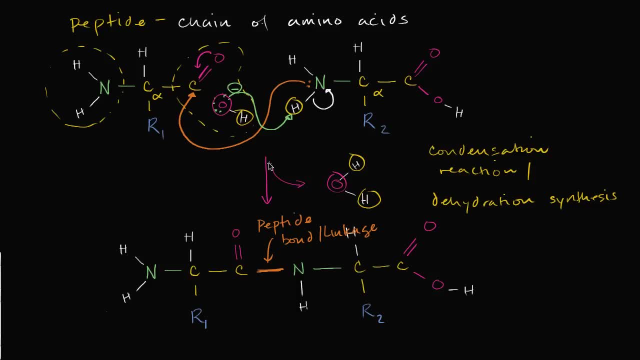 Now, when I first saw this reaction, I was like, okay, that kind of makes sense, Except for the fact that in at physiological pHs, amino acids don't tend to be in this form. In physiological pHs, you're more likely. 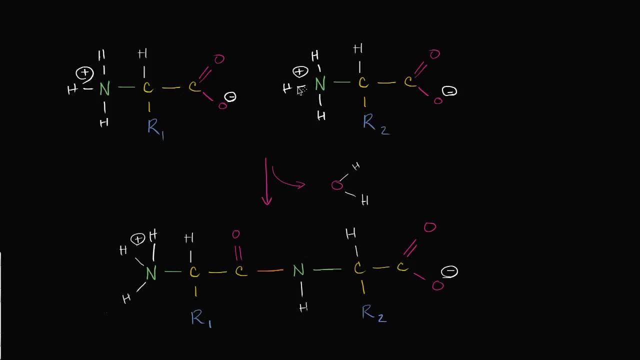 you're more likely to find this form of the amino acids. Define them as zwitterions or zwitterions, Zwitterions. let me write down that word. It's a fun word to say Zwitter. and it's one word, but I'm going to write. 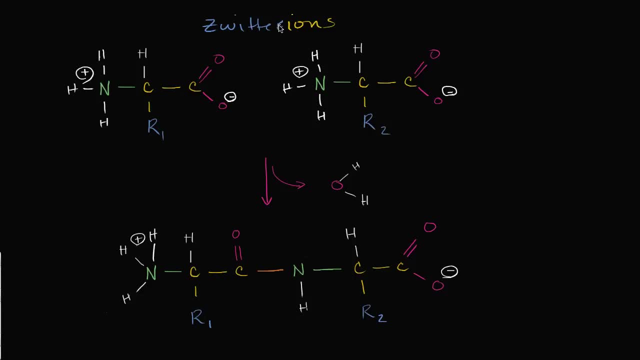 the two parts of the word in different colors so you can see it's saying it's a zwitterion. So what does that mean? Well, zwitter in German means hybrids. It's a hybrid. It's a hybrid ion. It's an ion. it has charge on different ends of it. 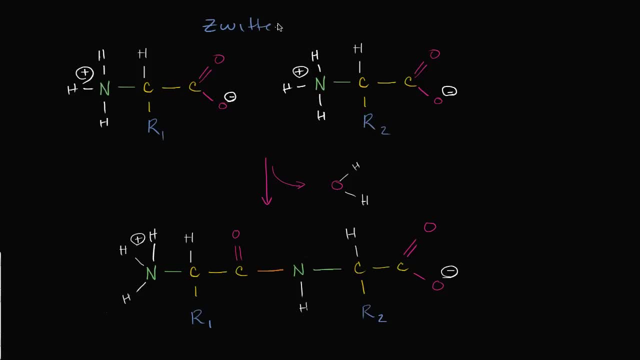 Zwitterions. let me write down that word. It's a fun word to say Zwitter and it's one word. but I'm gonna write the two parts of the word in different colors so you can see It's saying it's a zwitterion. 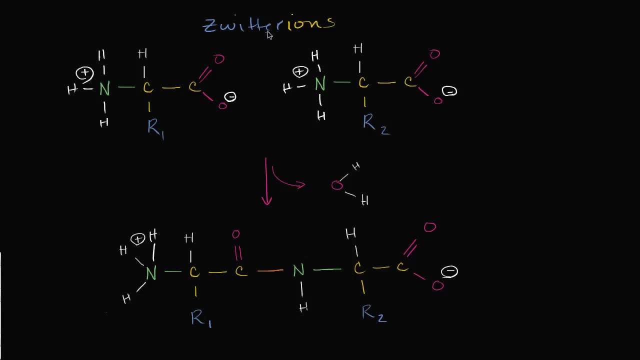 So what does that mean? Well, zwitter in German means hybrid. It's a hybrid ion. It's an ion. it has charge on different ends of it. It has parts of parts of the molecule have charge, but when you net them out you have it is neutral. 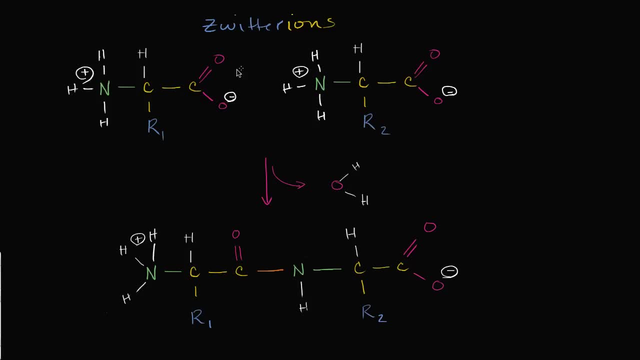 So they have. parts are charged, but it is neutral overall And so at physiological pHs the amino, the nitrogen end of the amino acid, tends to grab an extra proton, becomes a positive charge and the carboxyl group tends to let go of a proton. 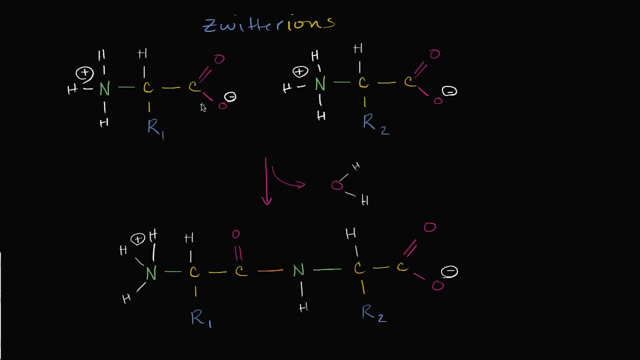 and has a negative charge. So this is your and this is actually going to be in equilibrium with the forms that we just saw before, but at physiological pHs it will actually tend to the zwitterion or the zwitterion form. 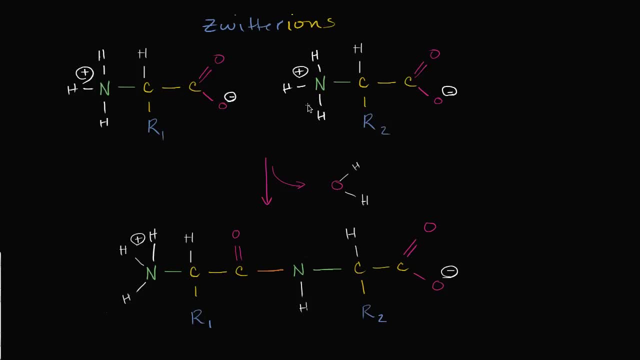 And so how do you get from this form to what to form a peptide bond? Well, you could imagine, you could imagine that this character over here, after giving its hydrogen protons, has an extra lone pair. So it's got. it's got: one lone pair, two lone pairs. 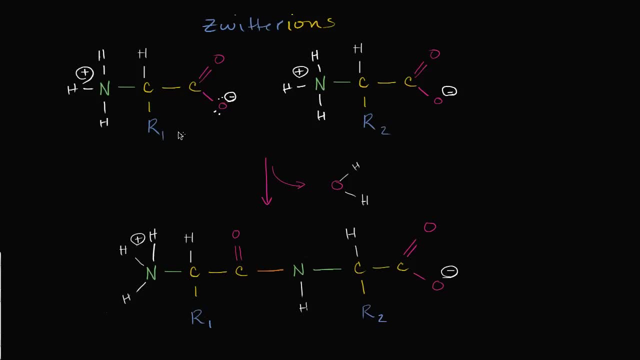 and then it's got. I'll do the extra lone pair and I'll do the extra lone pair in purple. It's got an extra lone pair. Well, maybe it could use. it could use that extra lone pair to either grab a proton from from the solution. 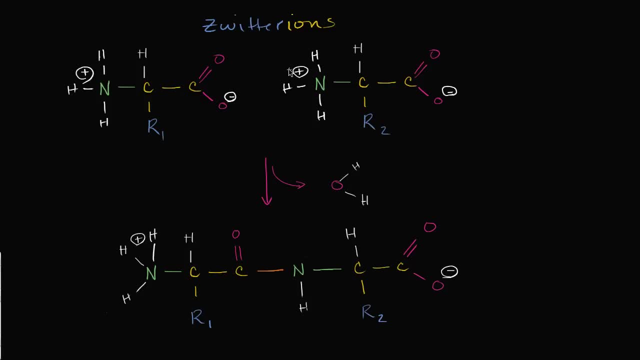 It has. parts of parts of the molecule have charge, but when you net them out you have it is neutral. So they have parts, are charged but it is neutral overall. And so, at physiological pHs, the amino, the nitrogen, end of the amino acid. 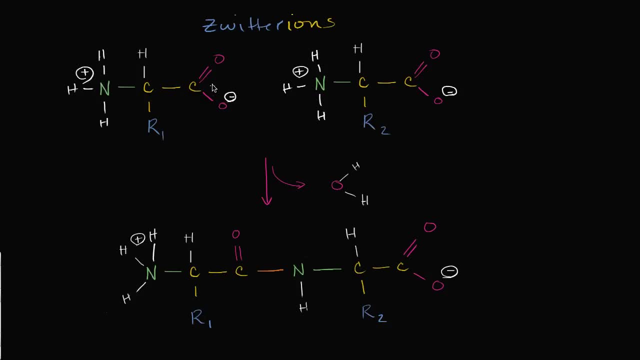 tends to grab an extra proton, becomes a positive charge, and the carboxyl group tends to let go of a proton And has a negative charge. So this is- and this is actually going to be- in equilibrium with the forms that we just saw before. 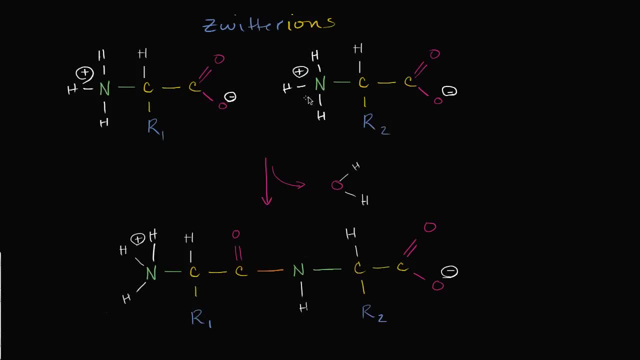 but at physiological pHs it will actually tend to the zwitterion or the zwitterion form. And so how do you get from this form to what to form a peptide bond? Well, you could imagine. you could imagine that this character over here, after giving 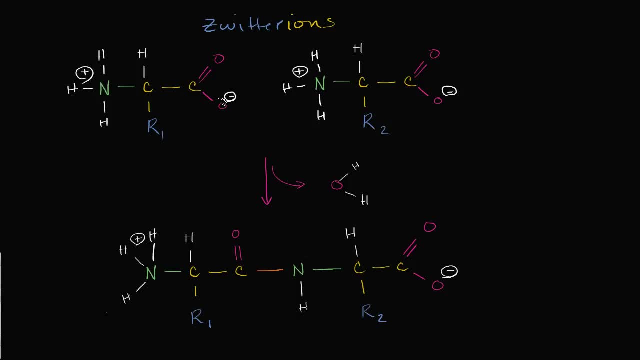 its hydrogen protons has an extra lone pair. So it's got. it's got one lone pair, two lone pairs and then it's got. this is: I'll do the extra lone pair in. I'll do the extra lone pair in purple. 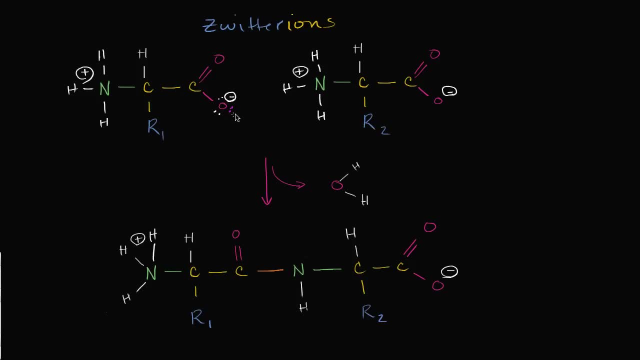 It's got an extra lone pair. Well, maybe it could use. it could use that extra lone pair to either grab a proton from from the solution or maybe just for for accounting convenience. we could say, well, maybe it just bumps in the right way. 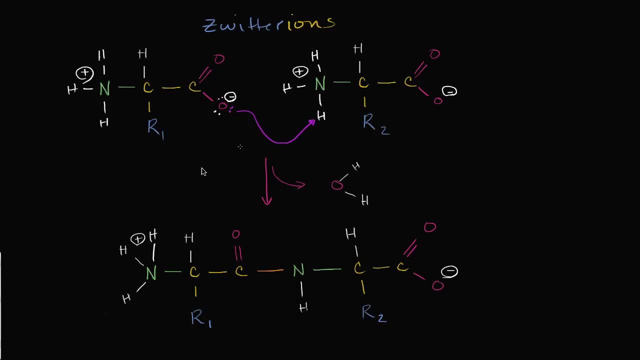 to grab this proton and then allows, and then allows the nitrogen, and then allows the nitrogen to take back these electrons. And if it did that, if it did that, well then you're getting, at least when you're looking at this carboxyl group and this amino group, 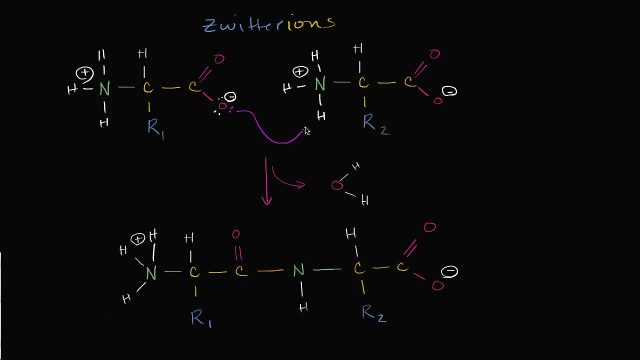 or maybe just for for accounting convenience. we could say: well, maybe it just bumps in the right way to grab this proton and then allows, and then allows the nitrogen, and then allows the nitrogen to take back these electrons. And if it did that, if it did that, 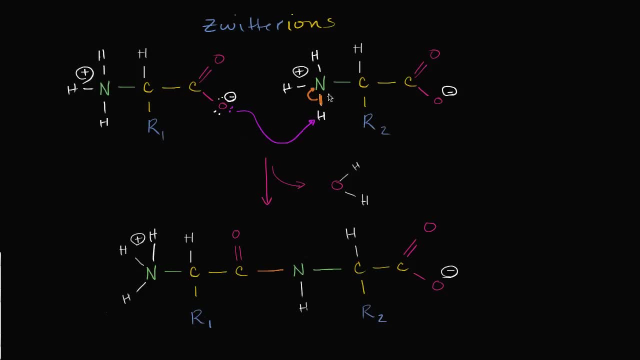 well then you're getting- at least when you're looking at this carboxyl group and this amino group, you're going to get to the form that we just saw. If this gets a hydrogen here, this is going to become a hydroxyl. 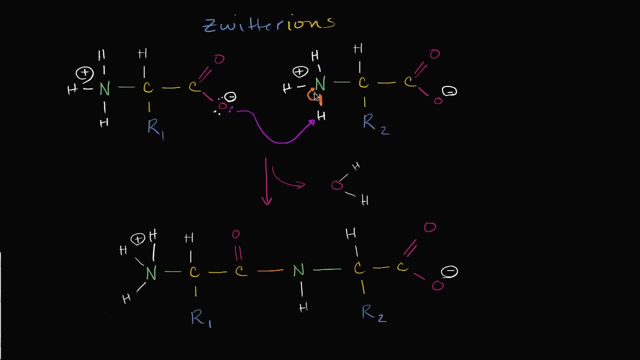 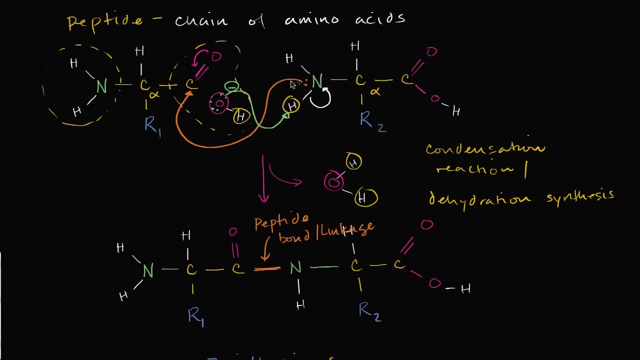 and if this, if this nitrogen takes back these two electrons from this pair, then it's just going to be NH2.. So it's going to be- it's going to be- at least this part of the molecules are going to be just what we started with up here. 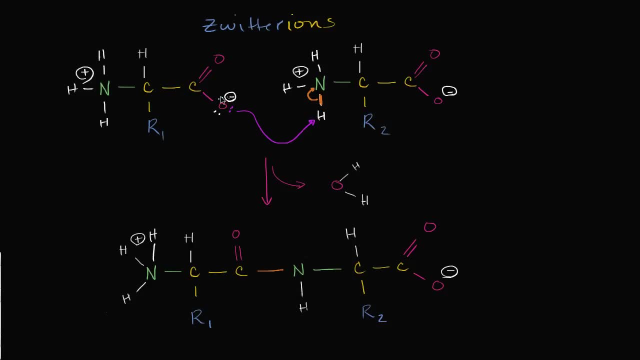 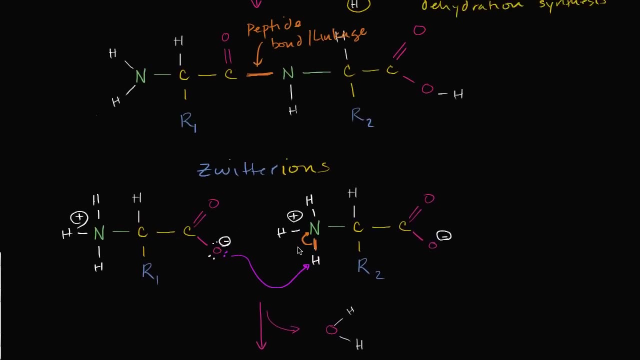 you're going to get to the form that we just saw. If this gets a hydrogen here, this is going to become a hydroxyl, and if this, if this nitrogen takes back these two electrons from this pair, then it's just going to be NH2.. 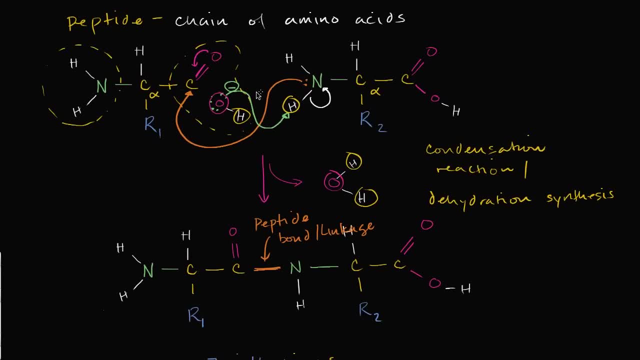 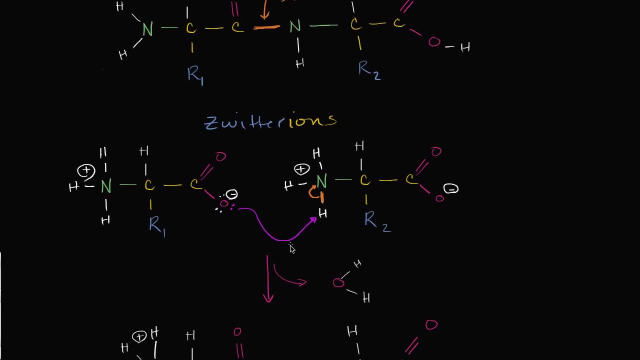 So it's going to be. it's going to be at least this part of the molecules are going to be just what we started with up here, And so you can imagine how you get back to the peptide linkage. The peptide linkage which we have right over here. 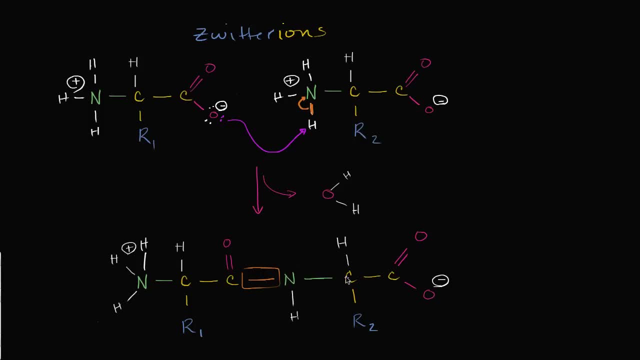 this is the peptide linkage, and then the only difference between the resulting, the resulting peptide that I have in this reaction- I guess you could say in the previous one- is: this is the zwitterion, the zwitterion form where this carboxyl group. I still have it.